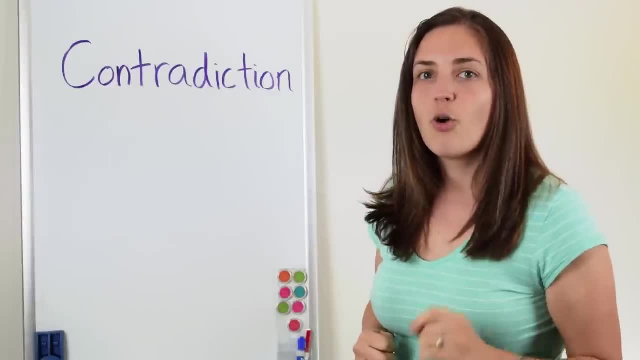 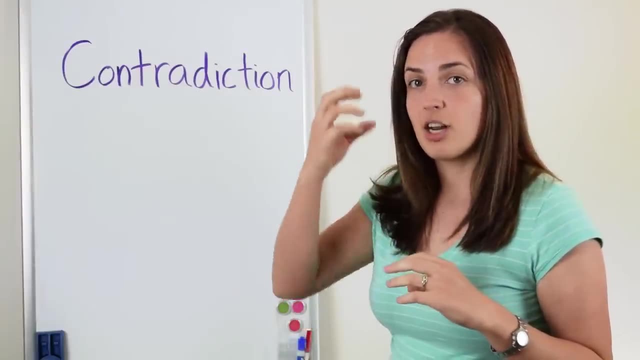 So, first of all, in order to explain what I'm going to prove, you need to know what a rational number is. So remember that a rational number is any number that can be written as a fraction of an integer divided by another integer. So let's write down what this is. 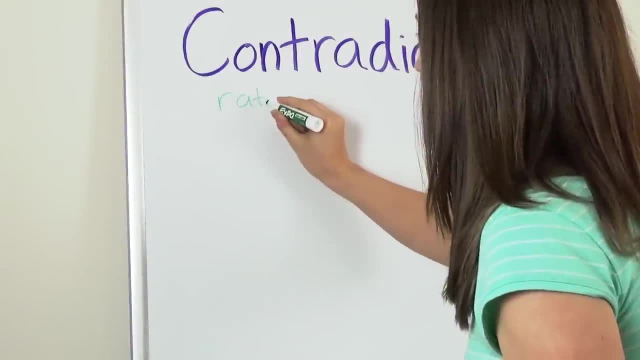 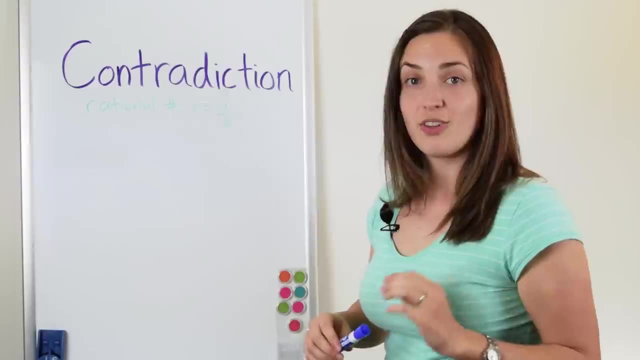 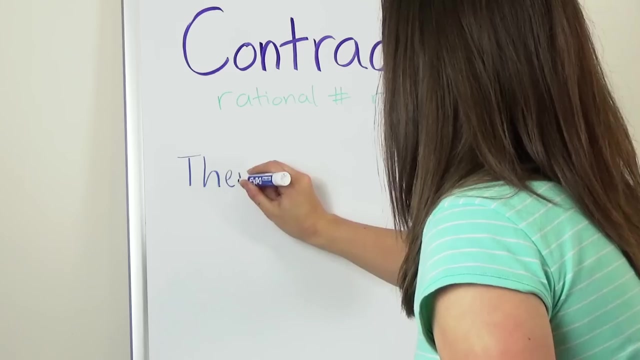 Rational number. Rational numbers are things that can be written down as a ratio, like a divided by b, where a and b are integers. So let's write down the statement that we want to prove: There is no smallest Rational number greater than zero. 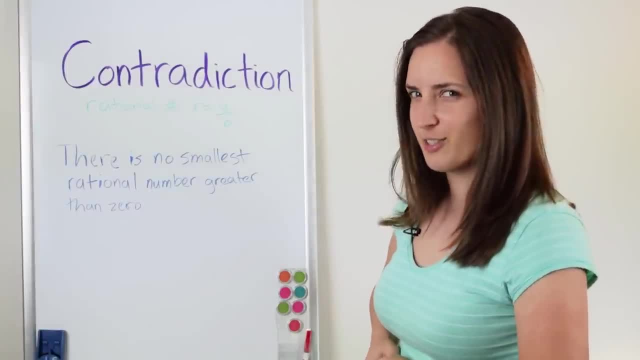 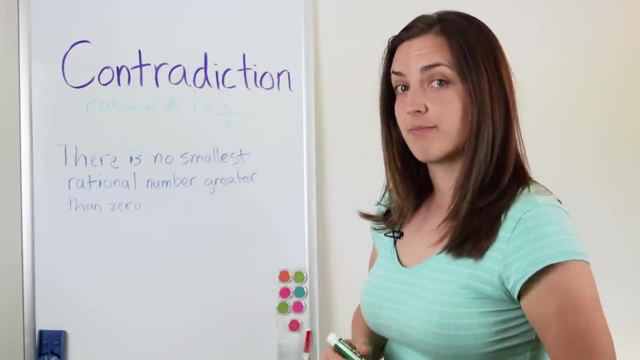 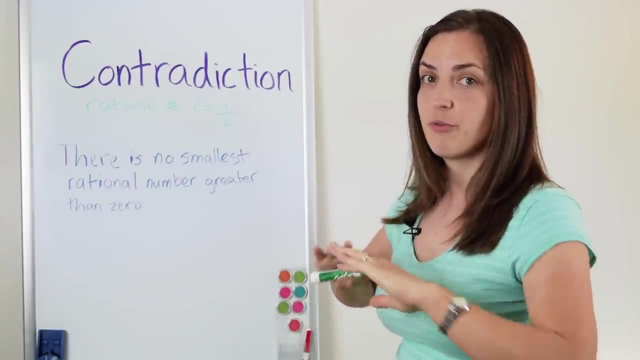 Interesting, right? You might think: sure I can find a smallest rational number, but you can't. And here's the proof. The proof goes by contradiction. So what we're going to do in a proof by contradiction is to assume that our statement, that we're trying to prove, is false. 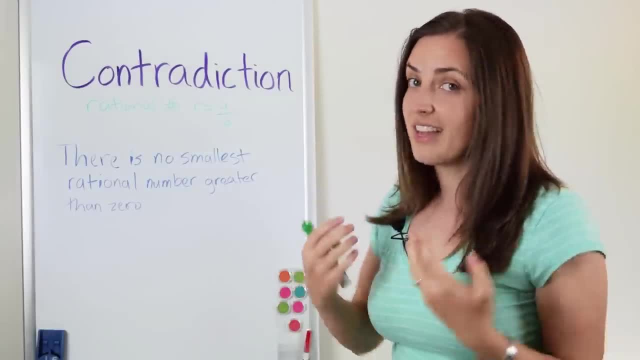 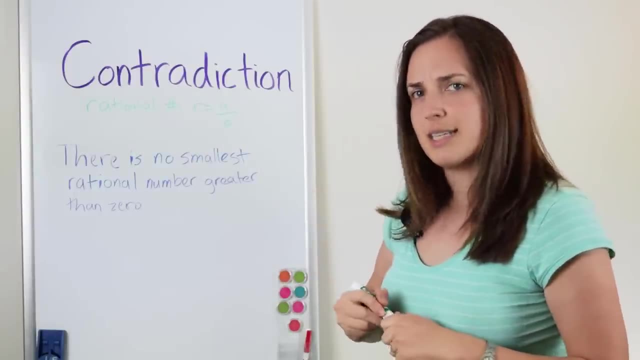 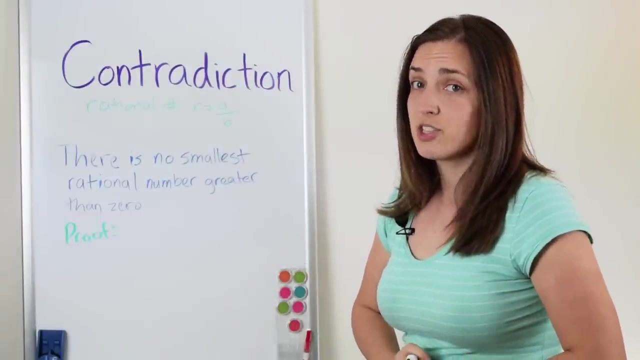 And then we're going to derive a contradiction and show that that's an impossibility. So what must have gone wrong? Well, our statement is false. Our statement must have actually been true. So let's work through the details, Proof In a proof by contradiction. we often start by saying, suppose not? 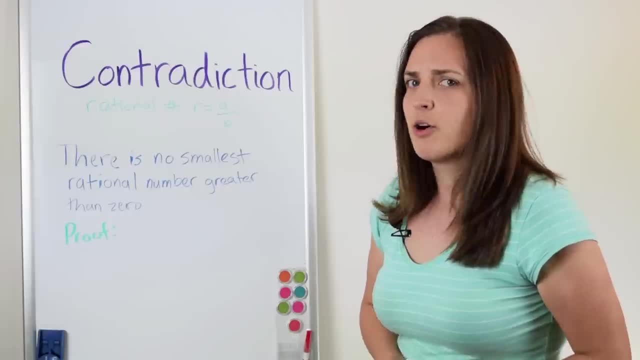 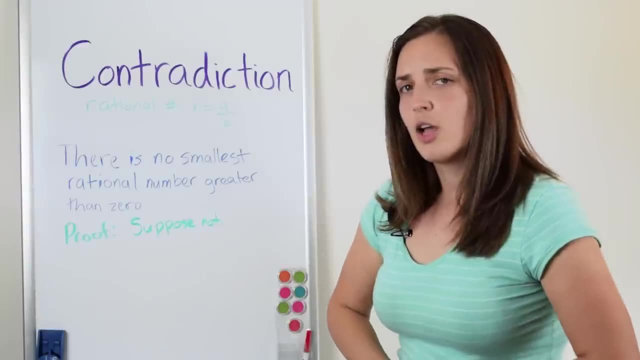 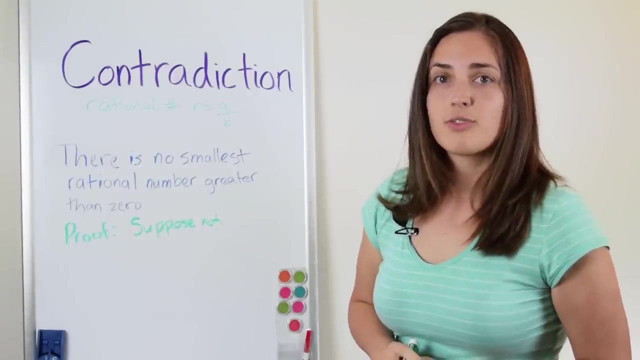 When we say suppose not, we really mean suppose that this statement we are trying to prove is not true. Okay, we've supposed that the statement is not true. That means that there is a smallest rational number bigger than zero, So let's write that down. 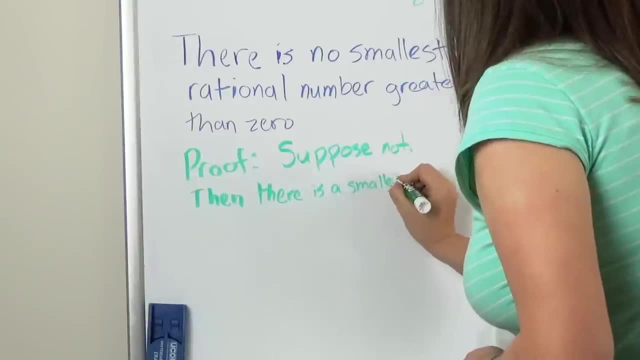 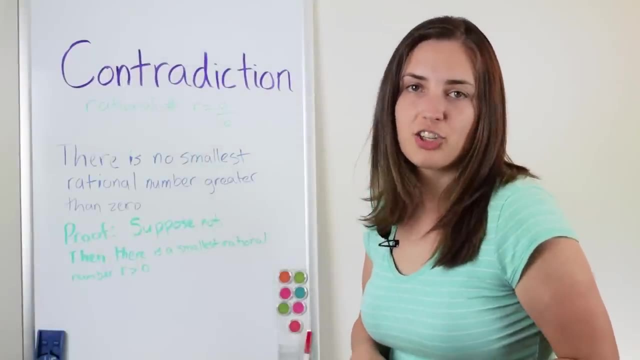 So then there is a smallest rational number. let's call it R, bigger than zero. Fair enough, So now we have our smallest rational number. But what can we do with this rational number? It's a fraction, It's sum A divided by sum B. 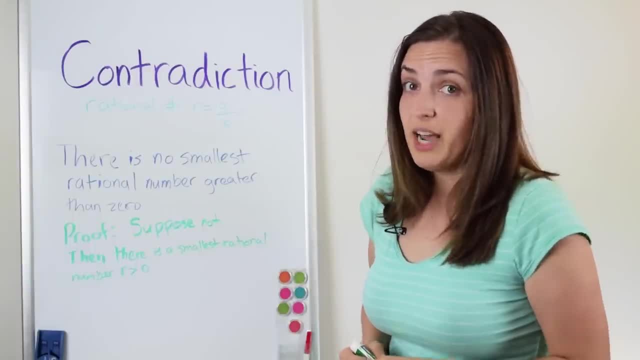 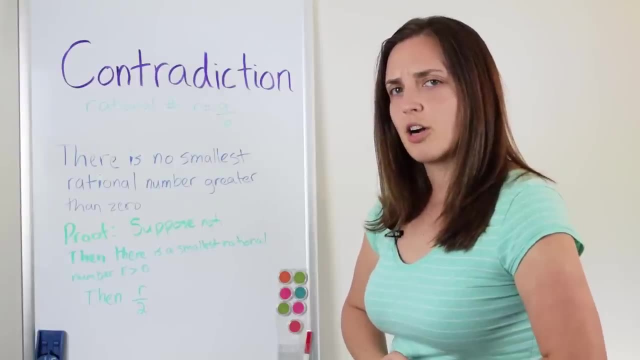 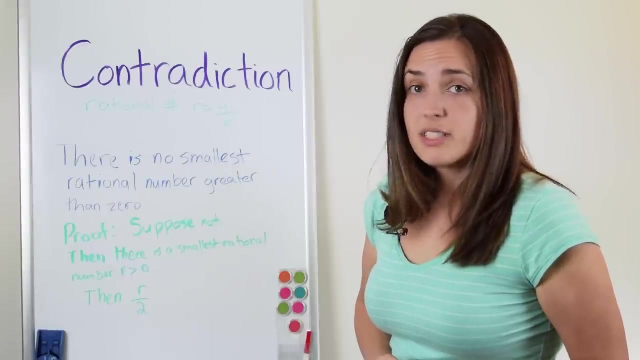 Why don't we take R and divide it by two? Let's see what happens. Well, what is R divided by two? If you have a rational number and you divide it by two, it's still a fraction. So R divided by two is a perfectly good rational number.